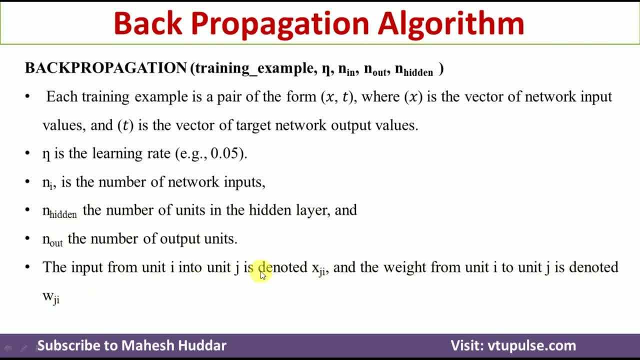 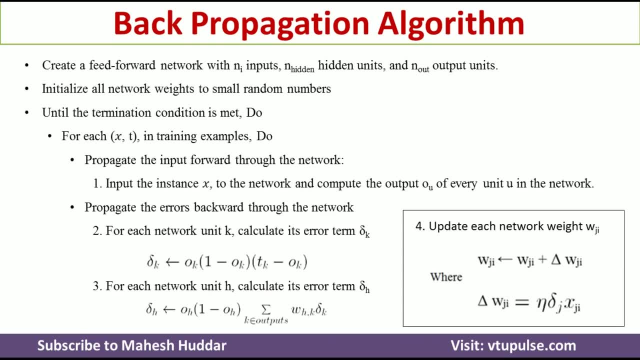 denoted as wji. We will see this particular thing when we construct a network in the next slide. This is the entire algorithm of back propagation algorithm. First, we need to create a feed forward network with ni inputs, n hidden units and nout output units. 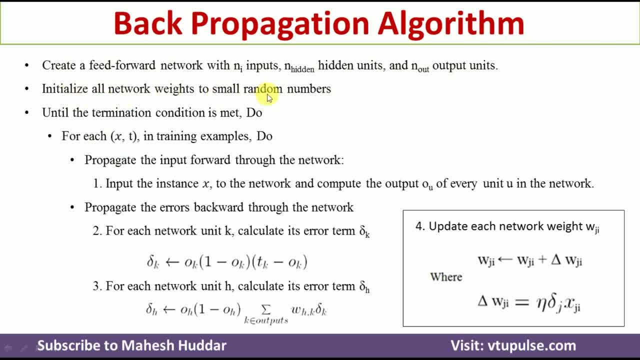 After that we need to initialize all the network units to a small random number. First we will see how to create a feed forward network with these number of units. For understanding purpose I have taken ni is equivalent to 3, that is. 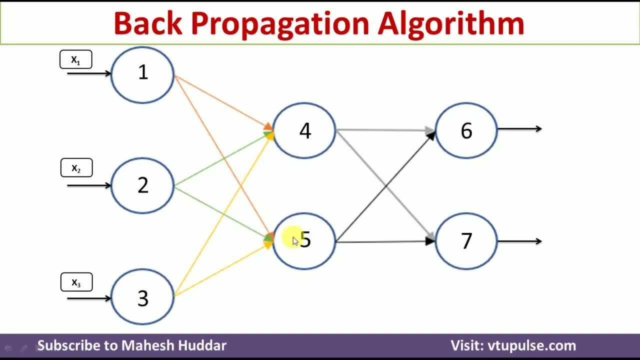 three units in the input layer: n hidden is equivalent to 2,, that is, two hidden layer units, and nout is equivalent to 2,, that is, two output layer units. in this case, x1,, x2, x3 are the inputs. 1,, 2,, 3,, 4,, 5, 6, 7 are the units in this case. 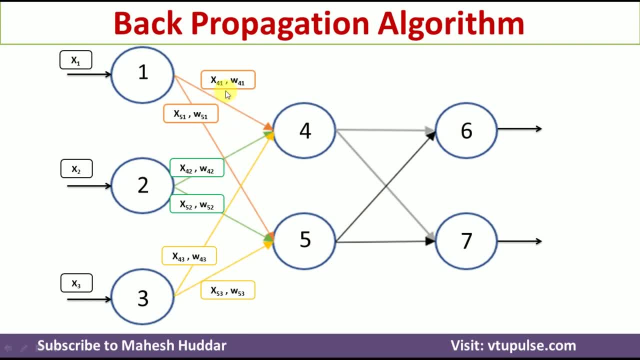 Next we need to assign the weights as well as the inputs. here The input from unit 1 to unit 4 is denoted as x41, that is nothing but x1 in this case. So x1 is known to us, that is. 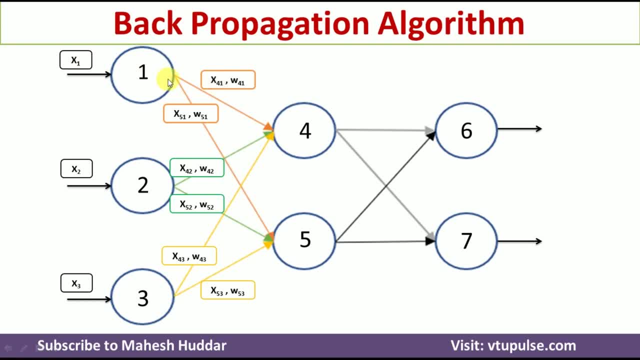 x41 in back propagation algorithm. Similarly, weight from 1 to 4 is denoted as w41.. With the same note, the input from unit 2 to unit 4 is denoted as x42 and the weight is denoted as. 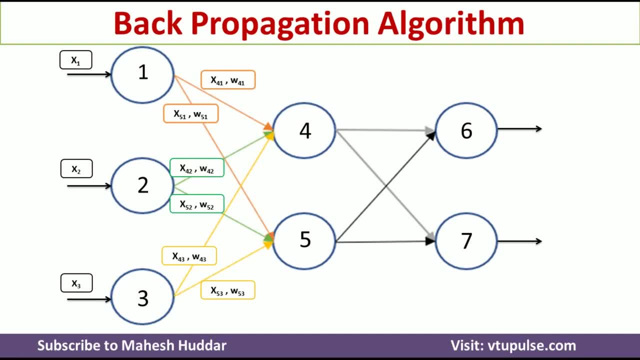 w42. in this case, The same thing goes with all the edges over here. Now we need to assign some input and weight to these particular edges. also, The weight from unit 4 to unit 6 is w64.. Similarly, input is x64.. The same thing goes with all the edges here. Now, in this case, we know. 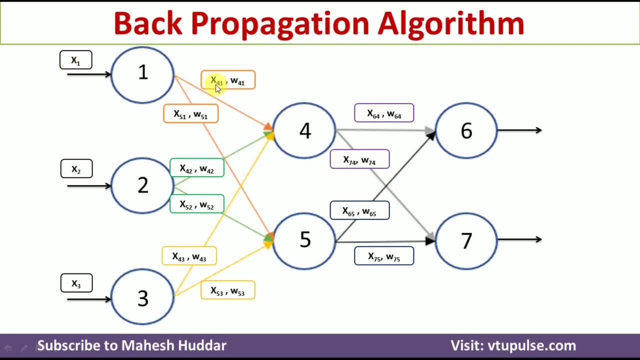 what is the value of x1.. The same thing is assigned to x41, x51. And we know the value of x2, that is assigned to x42 and x52.. x3 is known to us. that is assigned to x43 and x53. But we don't. 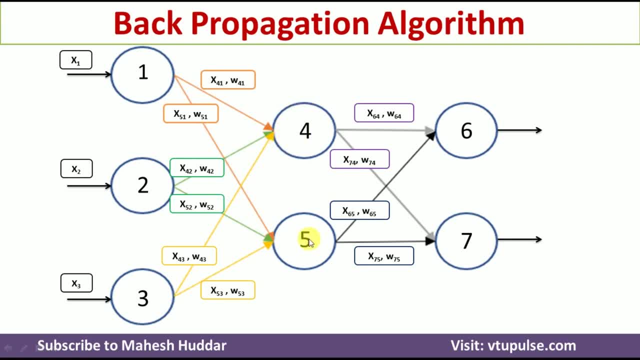 have any value or direct input to this unit 4 and 5.. So we don't have any values to x64 and x52.. x64, x74, x65 and x75. so what we do here is we will calculate the output of these units and 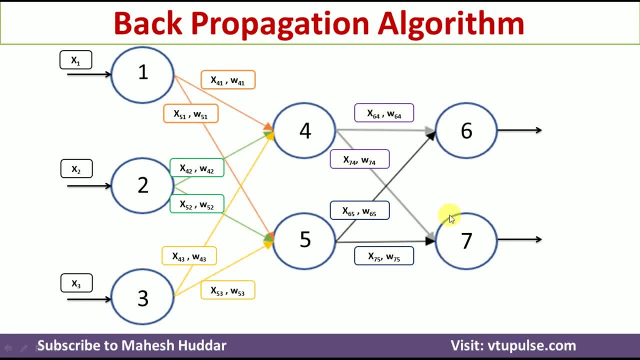 those output will be given as an input to this particular 6th and 7th unit and finally we will come up with the output here, that is, o6 and o7 are the outputs over here now. this is how we can construct the feed forward network. once you construct it for every weight we need to assign. 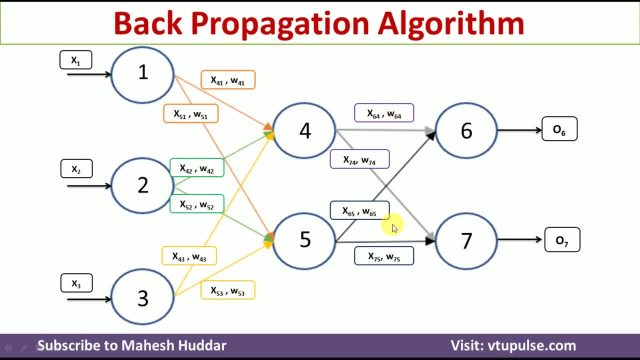 some random weights. you can assign any value in the range of minus 1 to plus 1. it should be a very small number. randomly, we need to assign the weights and in every iteration we go on modifying these particular weights unless and until we are happy with these particular outputs here. 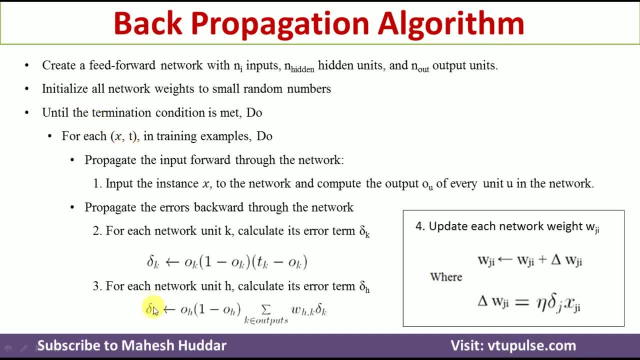 next is: we need to perform these particular four steps until the termination condition is satisfied or met. that is, the termination condition may be the number of epochs you need to perform these particular four steps. let us say that some 50- number of times that is the number of epochs. or you want to perform these particular four steps. let us say that unless and 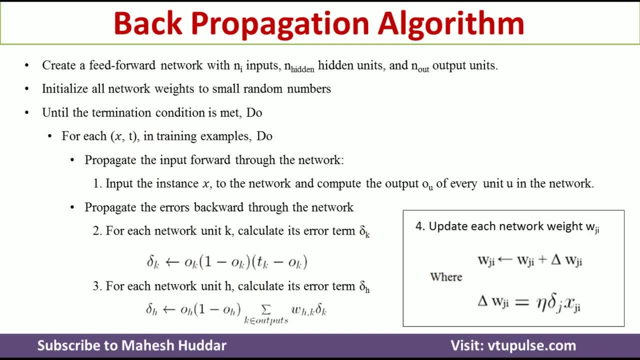 until you satisfied with the error rate. maybe let us say that you are expecting an error of less than 5 percent. unless and until you have error more than 5 percent, you need to perform these steps. once you achieve the error which is less than 5 percent, you can stop it so that 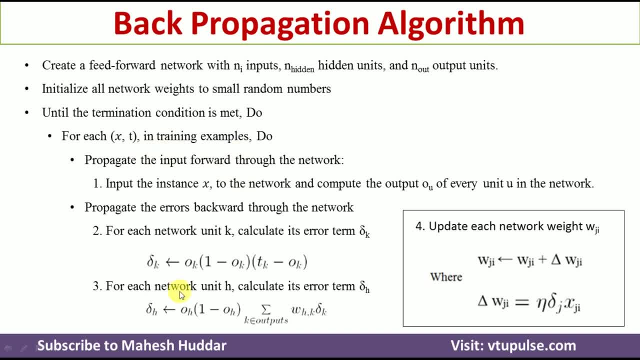 is one example here. now, what to do in this particular step is for each x comma t, that is, for each training example, we need to perform these steps. so what is that? we do? propagate the input forward through the network, that is, input the instance x to the network and compute the output. 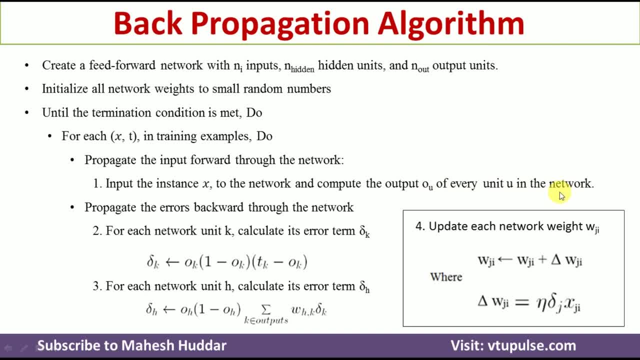 ou for every unit u in the network. that is, you need to give each instance to the network and you need to calculate the output of every unit in the network. i'll just show you that particular thing, how it will be calculated. first, what we need to do is we. 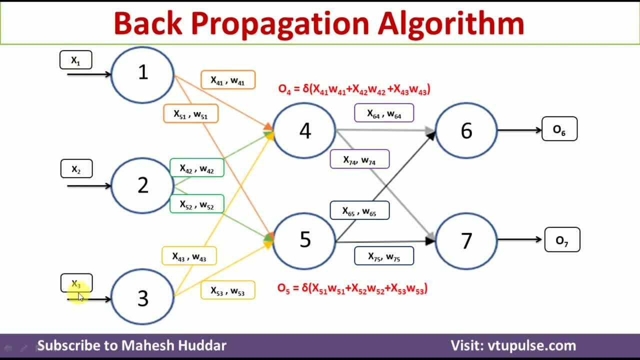 have these input and weight vectors. input is directly given from the instances and weight is assigned randomly. here we need to take these particular things and then we need to calculate the output of the fourth unit and fifth unit. that is the first unit of hidden layer and the second. 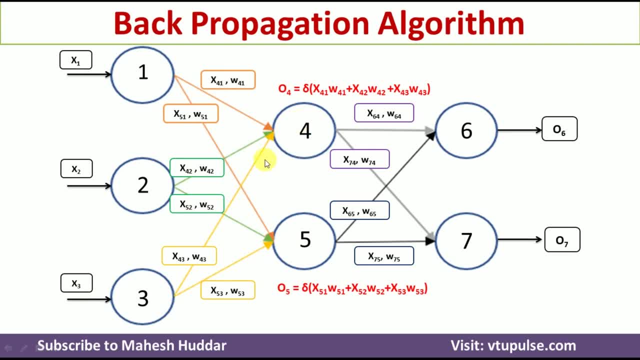 unit of hidden layer. so how to calculate it? to calculate this particular thing, we need to take the summation of linear combination of weight and input here. that is first to this particular node. that is fourth node. we have three edges coming here. that is: the edge is coming from one, edge is coming from two, as 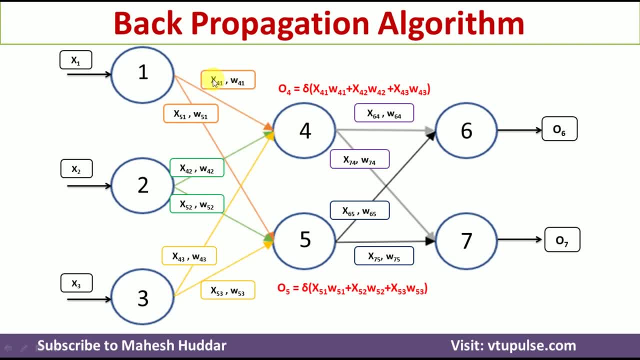 well, as edge is coming from three. so we will take the linear combination of weight and input and then we will take the sum of those things and finally we apply sigma term here. so how it is done is x 4 1 multiplied by w 4 1, plus x 4 2 multiplied by w 4 2. 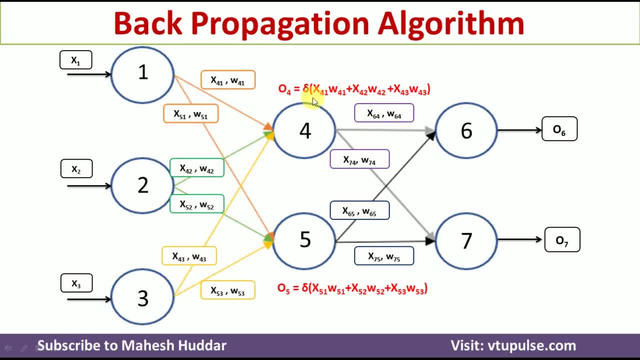 plus x, 4, 3 multiplied by w 4, 3, that is the summation term. once you get the summation term, we need to apply the sigma term here. sigma of x is always equivalent to 1 divided by 1 plus e raised to minus x. that is the sigma term. once you apply that particular thing, you will get the output at: 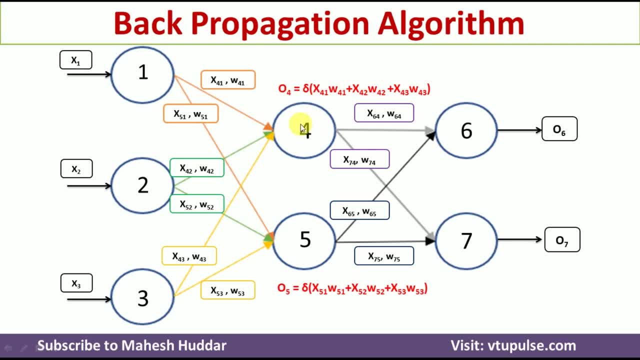 this particular node. so once you get the output at this node, we need to calculate the output at fifth node also. so again, we have three edges to this particular fifth node: uh, x phi 1 multiplied by w phi 1, plus x phi 2 multiplied by w phi 2, x phi 3 multiplied by w phi 3. so first we need to 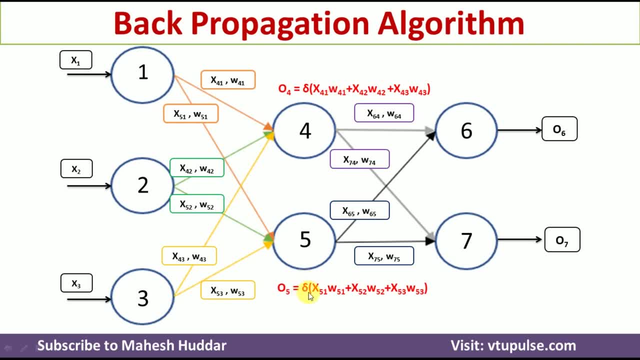 calculate this summation term and then we need to apply again: what the sigmoid? here the sigmoid is always equivalent to. i just write that particular equation here: uh, the sigmoid of x is always equivalent to 1 divided by 1 plus e raised to minus x. so whatever the value you get, i put that. 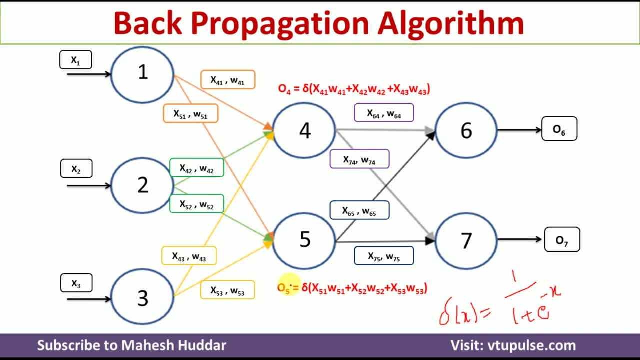 particular value in this x, you will get the sigma term, so you will get the output here. that is the what actually i am trying to say. so once you get this particular output at the unit number four and unit number five, they will be the input to this sixth and seventh unit. so o7 is uh, o4 is. 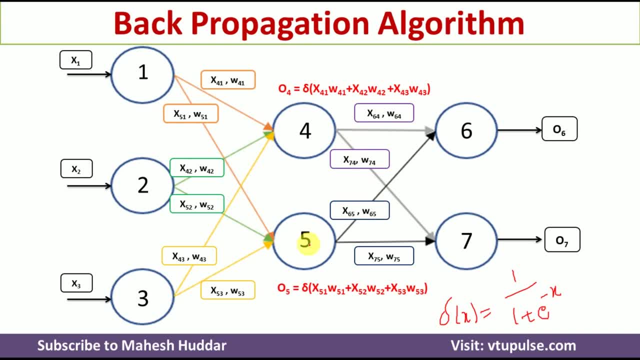 input to this particular edge and this edge and o5 is input to this edge and this edge here. so how it is denoted: uh, it is something like this: x64 and x74 is nothing, but uh, o4, uh, x65 and x75 is nothing. 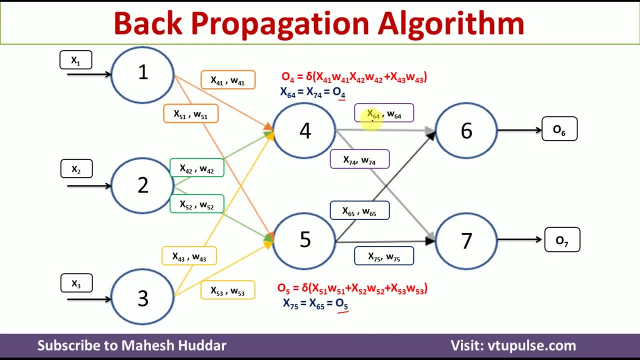 but o5 here. now you you know the value of x64, x74, x65, x75, and we have already assigned random weights to this particular thing. we will use the same technique, that is, we will take the linear combination of weight and input and then the sigma term to get the output at sixth node as well as. 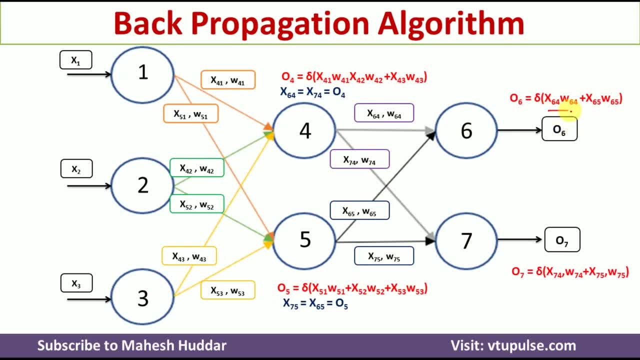 seventh node. so that is what we have done here. this is the linear combination of weight and input, and then we will apply the sigma term. we will get the output at sixth node. so that is nothing but the output here. similarly, we will perform the linear combination of weight and input and then sigma term to get the output at seventh node. so this: 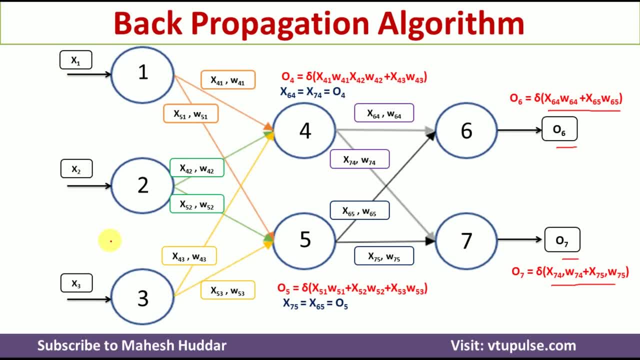 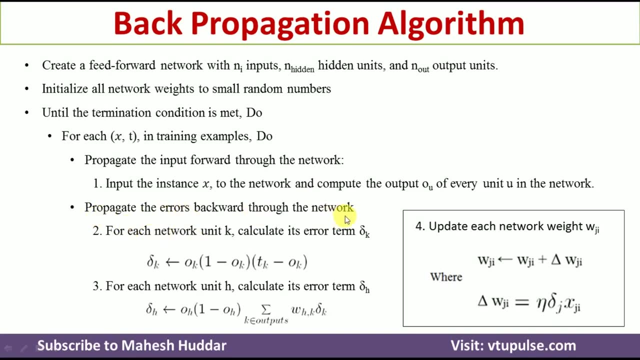 is how we will propagate the input- x1, x2, x3- till we reach the output at the end node. so this is the simplest procedure of propagating the input to get the output. here the next step is to propagate the errors backward through the network. in this case, what we do is- we have already calculated. 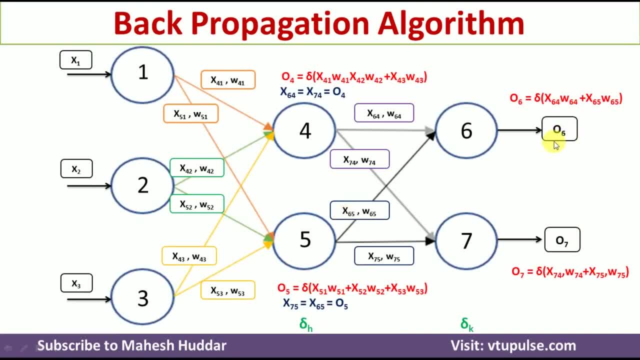 the outputs here. once you calculate these particular outputs, we need to calculate the error terms. once you calculate that particular error term, the error term is propagated to all the hidden layer units and using that particular error term, we will try to modify this particular weights here. so that is the thing what we do in this case. so what we do here is: first, we will 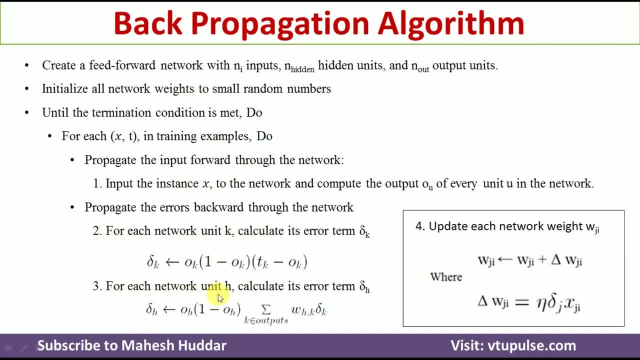 calculate the error at the output unit and then we will calculate the error at the hidden unit. to calculate the error at the output unit we use this equation. the equation in this case is: delta. k is equivalent to ok multiplied by 1 minus ok. multiplied by tk minus ok. here, where k is the 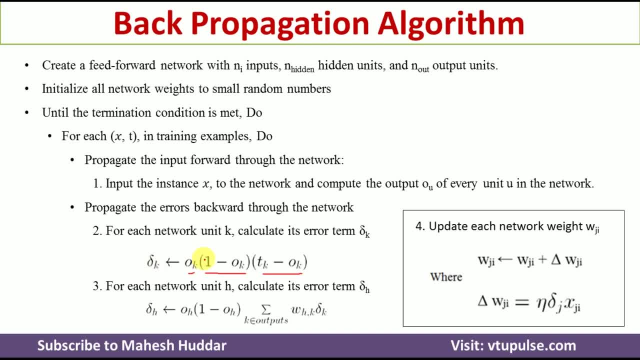 output unit number. for example, if you want to calculate the error at the sixth unit, it will be something like this: delta 6 is equivalent to o 6 multiplied by 1 minus o 6. multiplied by t 6 minus o 6, o 6 is the output and t 6 is the target. that is the expected output. 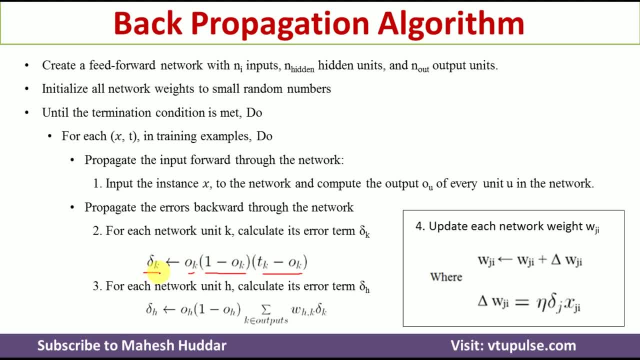 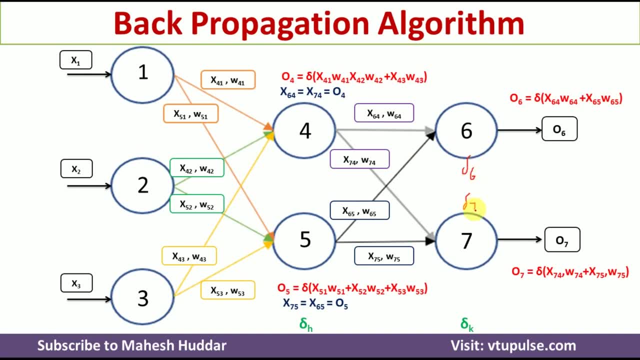 so, using these particular values, we calculate the delta 6. similarly, we calculate delta 7 also. so we calculate delta 6 here and then we calculate delta 7.. now, once you calculate these delta 6 and delta 7, one thing we need to notice here is this: delta 6 is due to the unit number 4 and unit number 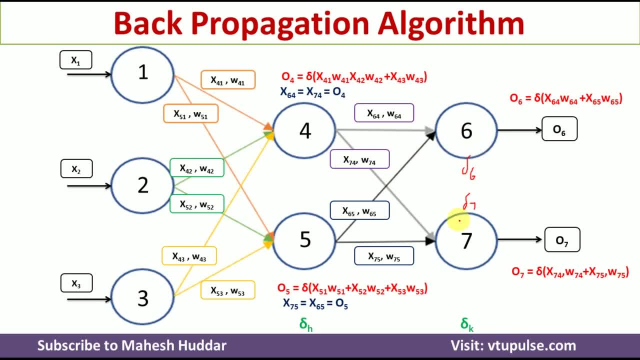 5, because these two edges are coming towards it. similarly, this delta 7 is due to unit number 4 and unit number 5.. so what we need to do is we need to propagate this delta 6 to unit number 4 and unit number 5, as well as delta 7 to unit number 4 and unit number 5 here. so how to propagate the 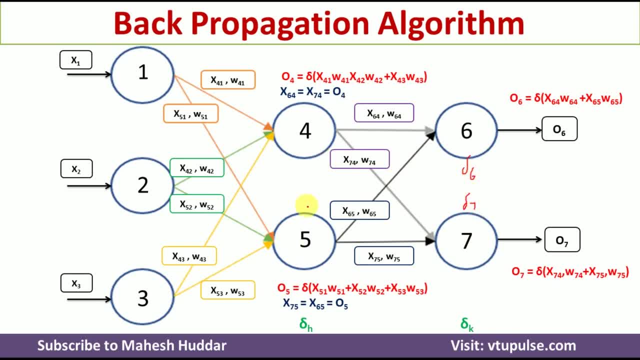 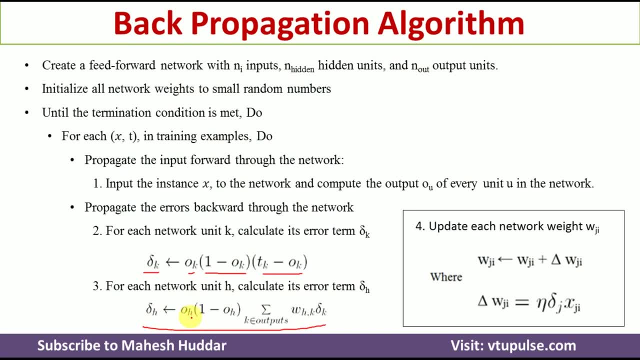 question is how to propagate this particular error backwards. to propagate that particular error backwards, we use this equation. in this equation we have: oh, that is, the output at hidden layer multiplied by 1 minus o, h, h- in this case you can take the first time- 4 and. 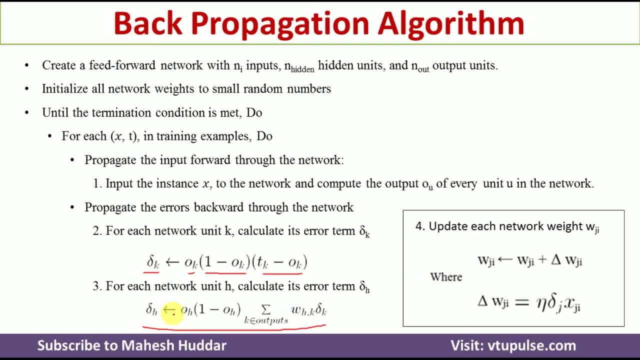 second time 5, so it will be: delta 4 is equivalent to o 4 multiplied by 1 minus o 4. o 4 is known to us. no issues this particular term here. what we are trying to do is we are trying to propagate this particular delta k backwards due to all the output units, because if you see here this particular 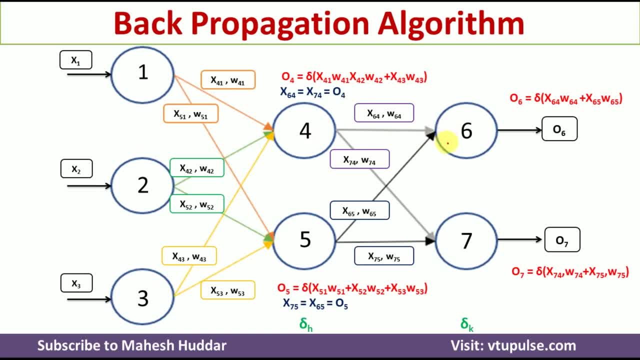 the error at 4th unit unit is due to the delta 6 also as well as delta 7 also. similarly for this one, delta 6 also as well as delta 7 here. so what we do here is we will use this particular delta 6 and 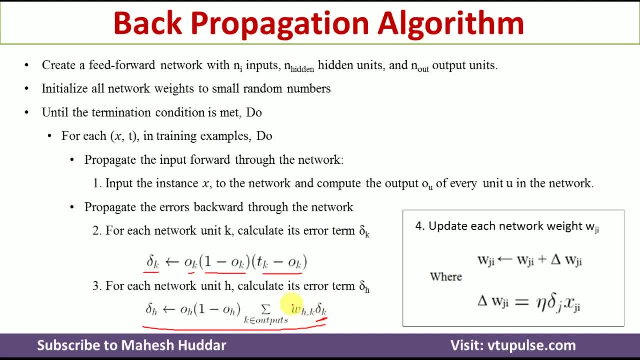 delta 7, both the units, and we will multiply the weight vector of that particular edge so that you will get the error at the hidden layer. so we do this particular thing two times because we have delta 4 and delta 5 to be calculated once you. 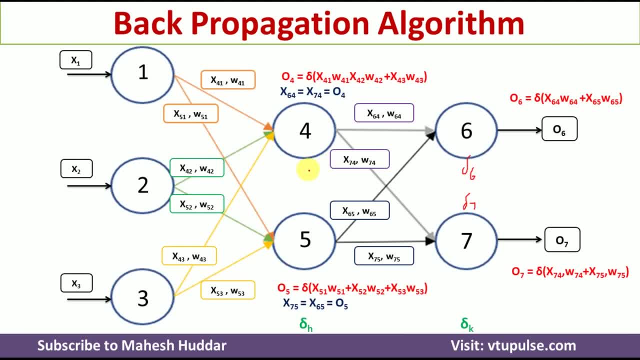 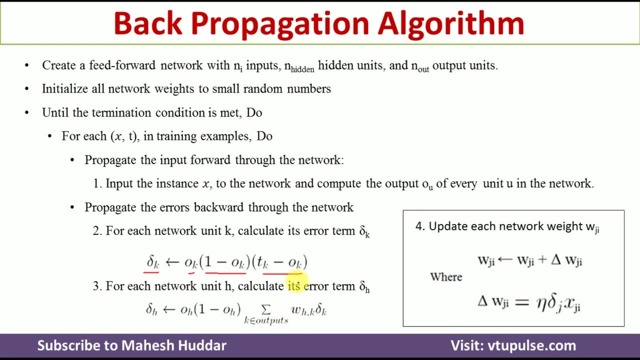 calculate that particular thing. we got the errors at the hidden layers also, that is, the delta 4 is available as well as delta 6. delta 5 is available here. so we have calculated the errors at all the units now. now the question is: how did we got these particular equations? these equations are to be: 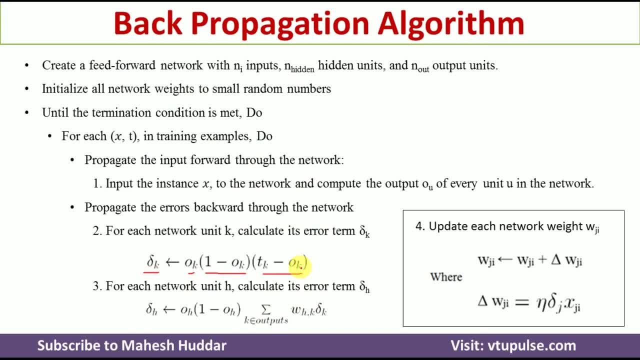 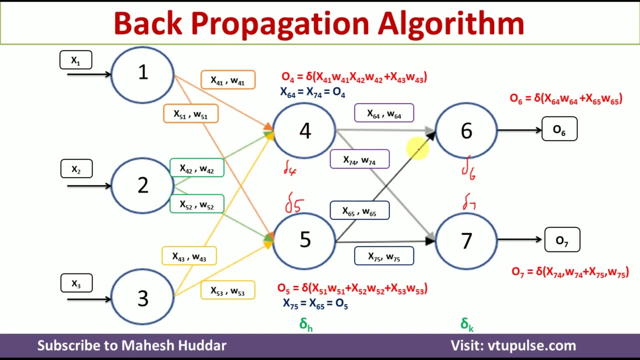 derived. i have already posted a video on this particular thing- how to derive these particular equations like delta k and delta h. link for that video is given in the description below. go through that particular video to understand how to derive these particular equations. here now we found the errors at every unit. the next step is to use these particular weights to update. 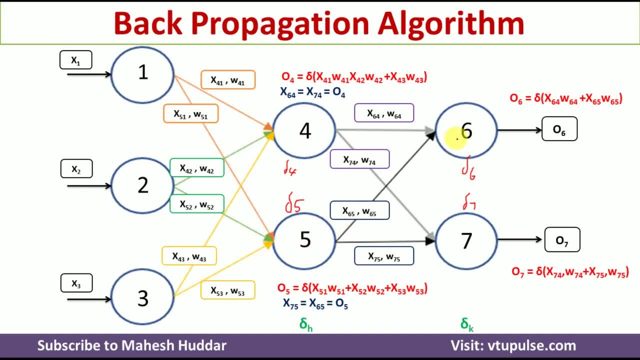 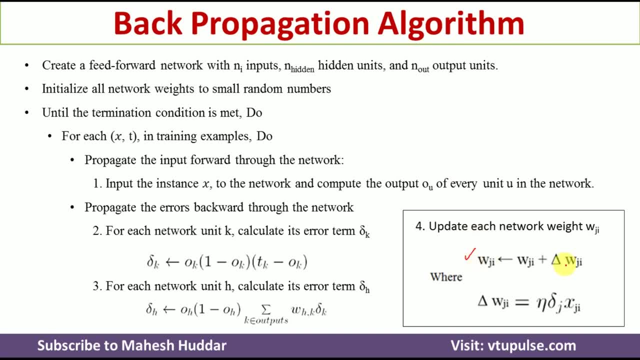 this particular weights in this case, usually the process is very simple. we use this particular equation: delta w wji is calculated and that delta wji is added to the current weight here, that is, wji is equivalent to wji plus delta wji. the question is: how to calculate delta wji? delta wji is calculated by: 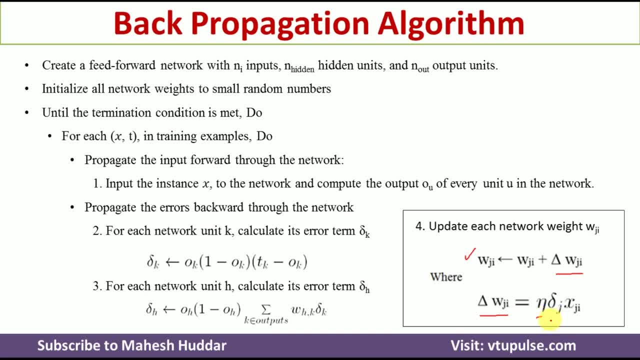 the learning rate. we know that particular value, delta j, that is error at each unit. we have already calculated, so we will multiply that and then xji. here xji is nothing but the input we use: the learning rate, the error of that particular node multiplied by, if you are calculating the 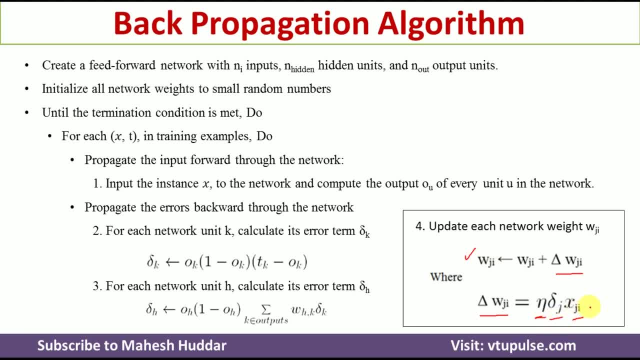 weight for wji. we use xji, that is input. using this we calculate delta wji and we add that particular thing to the current weight to get the new weight. here it may be the increment or decrement, but we add at add this thing to the existing weight to get the new weight, here the 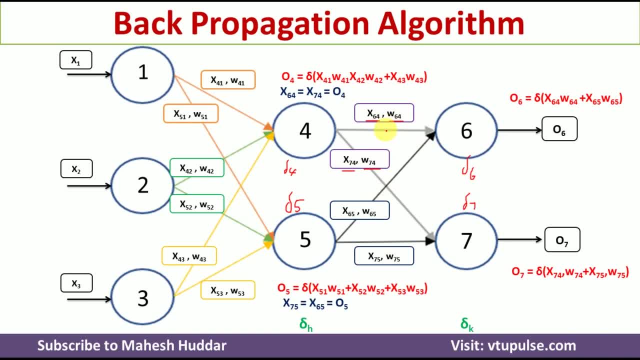 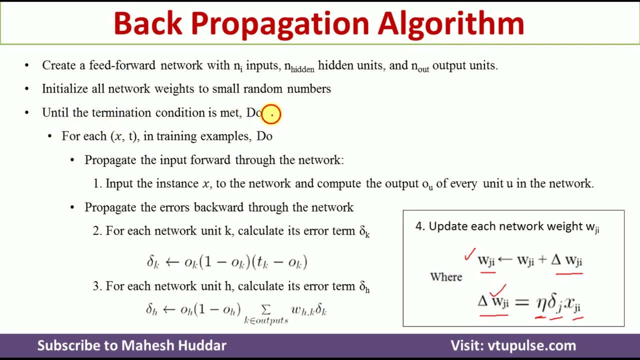 same thing is repeated for all the weights. these are called as output length layer weights and these are called as hidden layer weights. All these particular weights are calculated. Once you calculate these particular weights, next we need to go back to this particular step. We need to check whether the number of epochs are reached or we have satisfied with the. 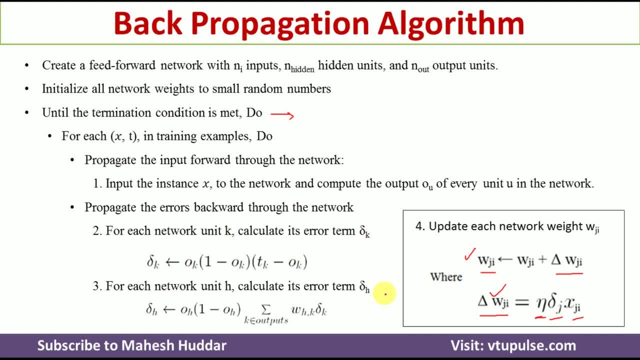 error. If not, we need to perform these particular steps again here. We need to propagate that input instance from input layer node to output layer node and then we need to calculate the error at the output layer. We need to calculate the error at the hidden layer Using these two error terms.